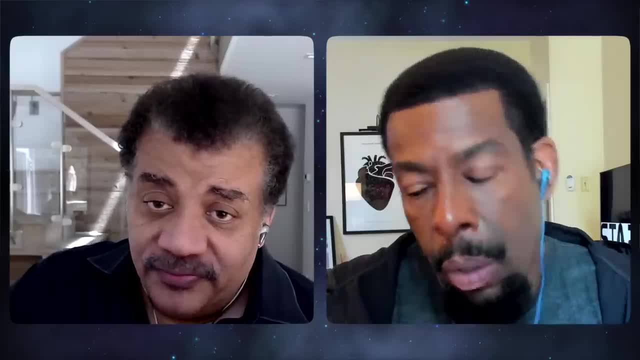 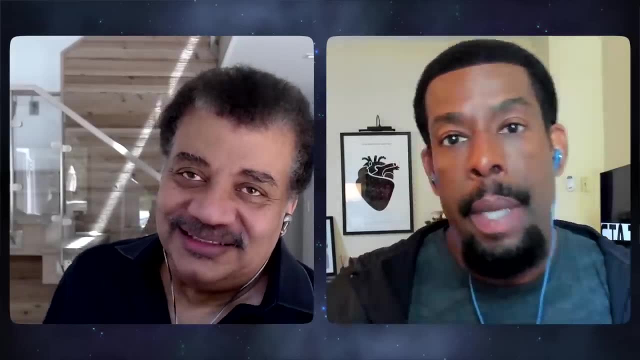 You're going to climb over the top of the hill and come down the other side. I mean, that's why I had children. They're going to pull me up over the hill. Let them do the work. I'm going to sit right here in this little cart. 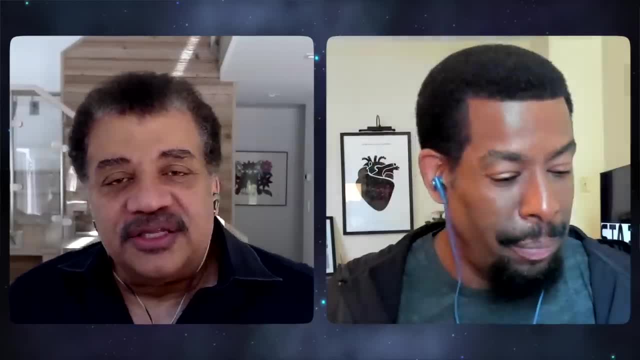 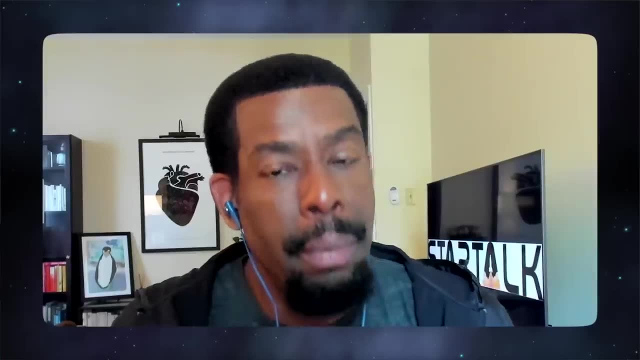 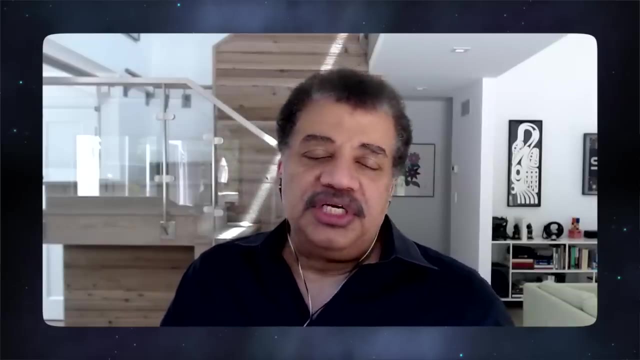 Y'all get moving. So another way to do it is to bore a hole through the mountain, through the hill, and come out the other side. So true, By doing so you've made a tunnel, Correct, Okay, So you've made it easier to get from one side of the hill to the other, because you don't have to go up and then come back down. 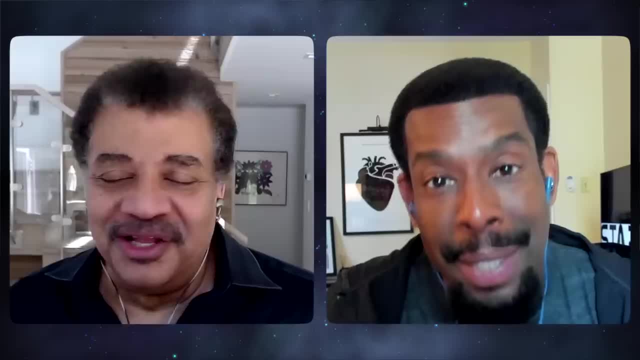 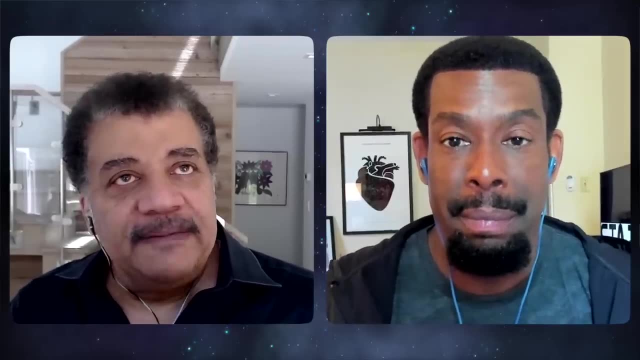 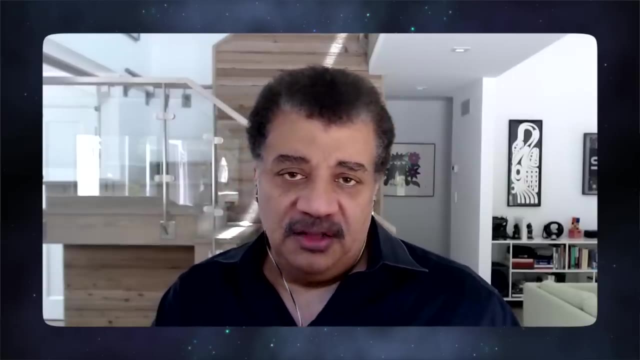 As a person who lives in Jersey, I appreciate that concept And the tunneling from out of Manhattan. That's right, Correct, Okay. So here's something interesting: In quantum physics, we can think of the hill as an energy barrier to you. 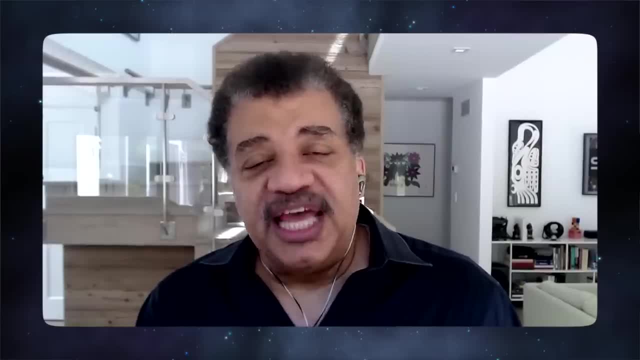 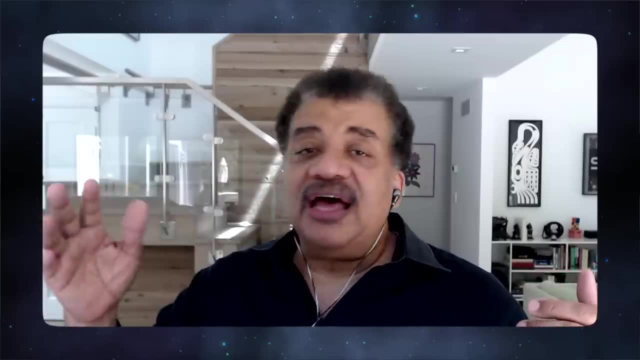 Okay. Okay, That makes sense. All right, So you need energy to ascend the hill, Otherwise you'll just stay where you are. So now we check: How much energy do you have? Oh, I can get halfway up the hill, but not any further. 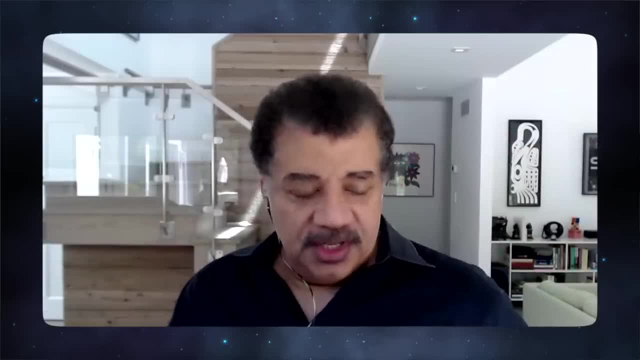 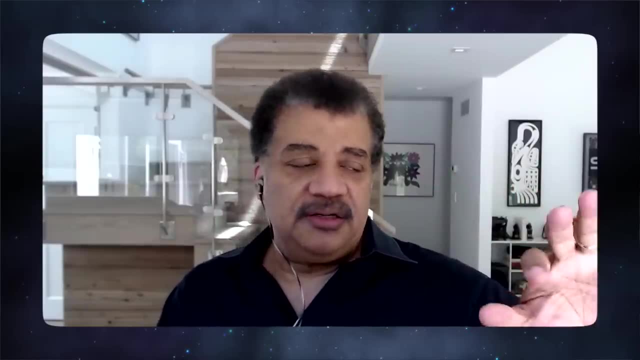 Three-quarters of the way, but not any further. Okay, So in quantum physics, if there's a hill, we call them potential barriers, because, all right, they're actual barriers, but they're called potential barriers. So there it is. 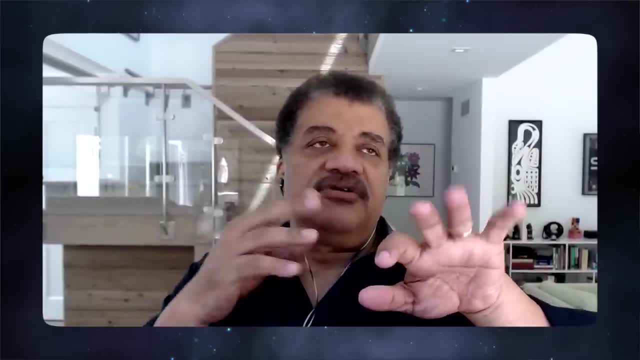 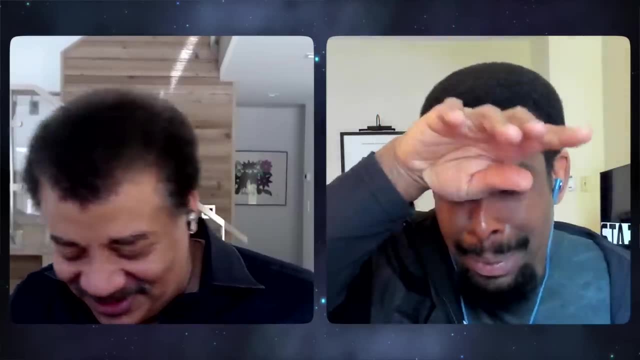 You have a particle on one side of that barrier And you give the particle energy. I can't make it. I can't make it. Okay, This hill is too much. Oh, Why you got to. Let's just stay here. 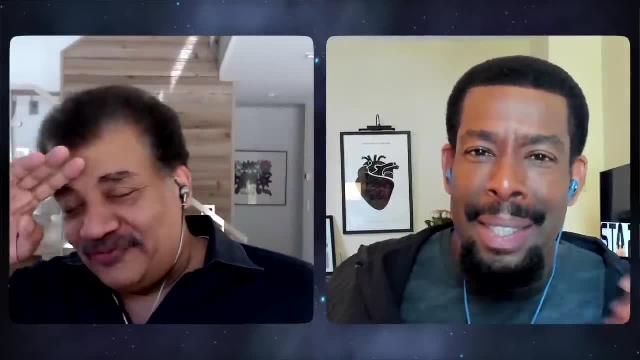 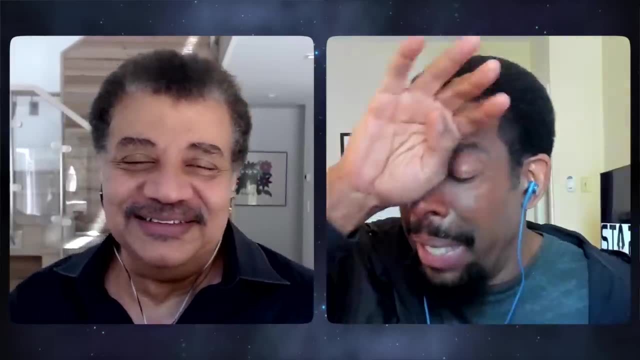 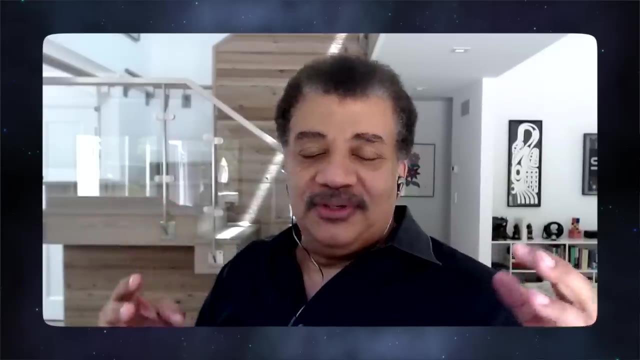 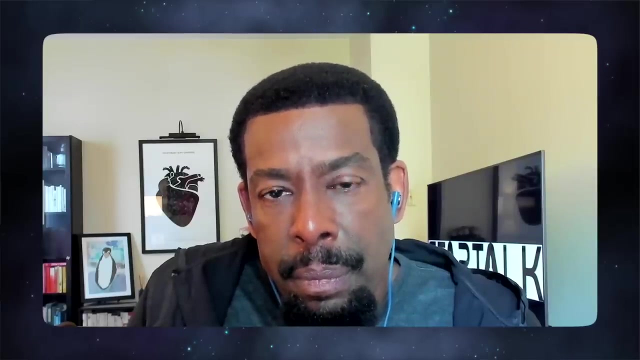 Why don't we just live here now? You're wiping the sweat off your brow like electron sweat. You have no idea how hot that nucleus. So the particle, however, is not only a particle, it's also a wave. Okay, And when you're a wave, there's something called a wave function. 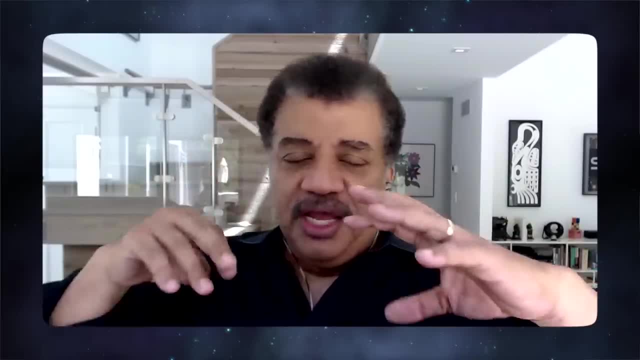 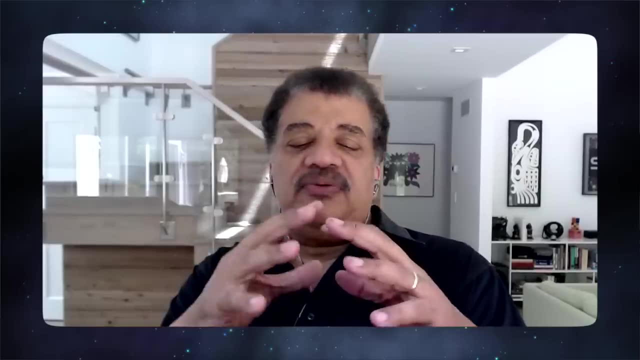 And a wave function is the probability of finding it anywhere in a volume spanned by that wave function. Okay, So you're more likely to find it where the wave peaks and where the wave drops off. you're less and less likely to find it there. 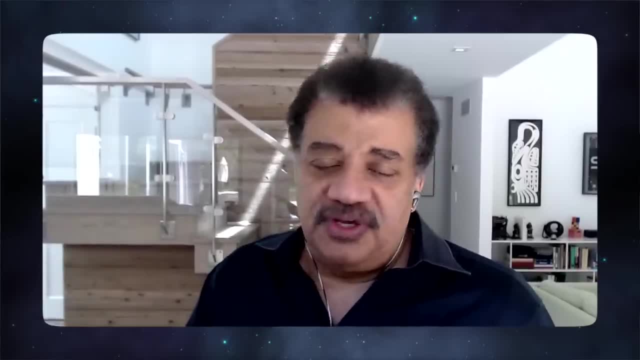 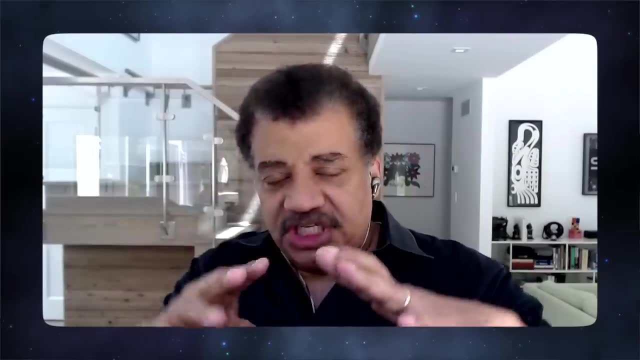 And there's a point where don't ever wait around because it won't show up for trillions of years. All right So, but there's an actual likelihood. it can show up anywhere in the wave function, even in the low probability places. 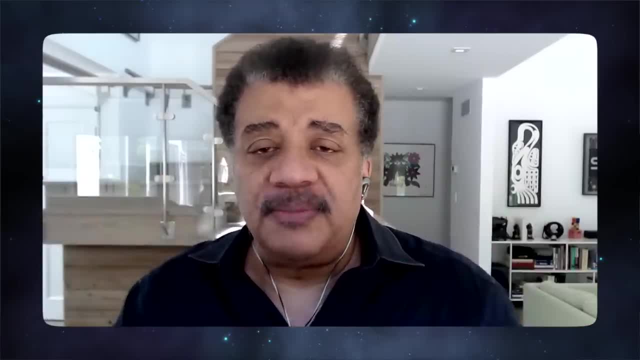 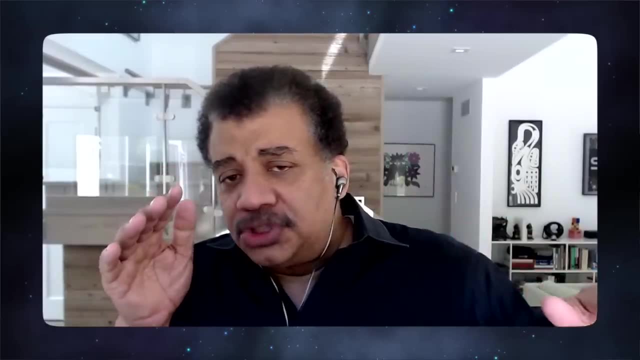 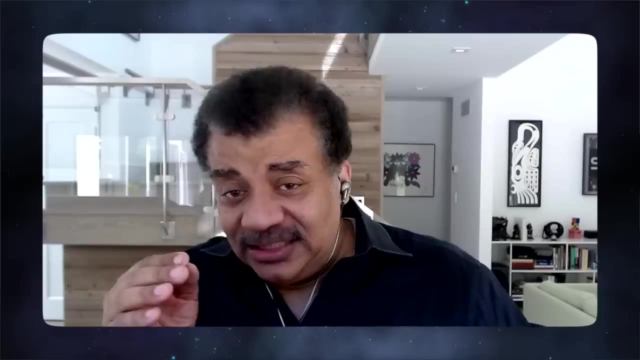 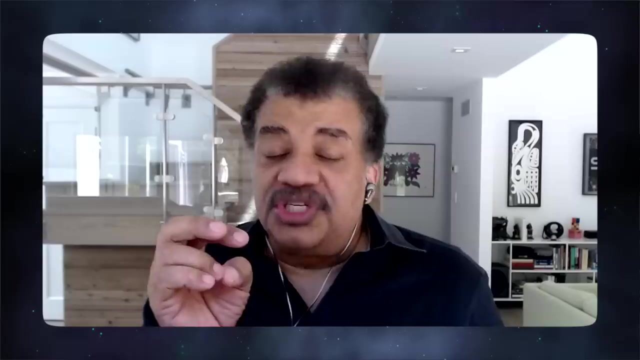 All right, So that wave doesn't. It doesn't know about and doesn't care about the mountain. Okay, So you can ask: does some of that wave show up on the other side of the mountain? Aha, If it does, then there is a probability that the particle that's stuck on one side will just simply appear on the other side of the mountain, having never had to ascend it in the first place. 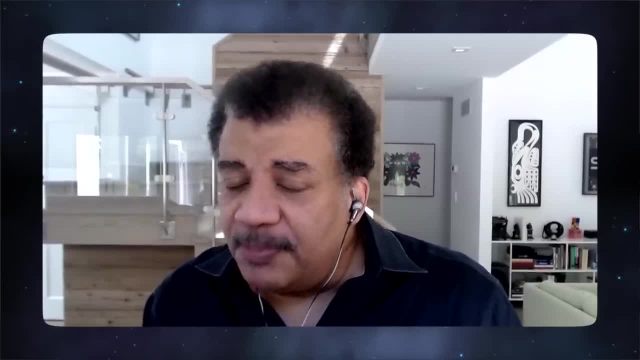 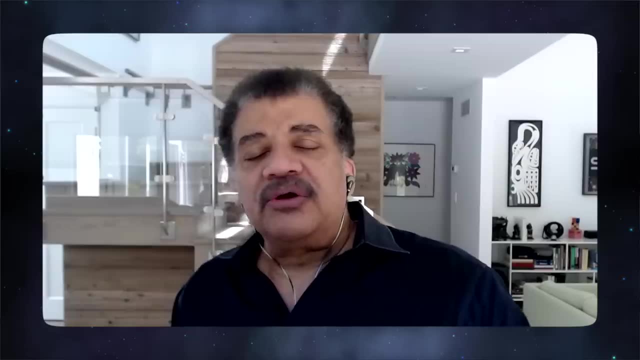 Okay, Okay, Okay, Okay, Okay. So it didn't have enough energy to do it, But because it exists as a wave function, there will always be a probability that it can show up where it was not invited. Oh, That's called quantum mechanical tunneling. 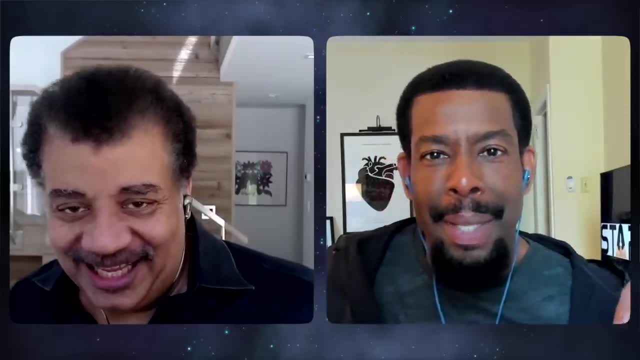 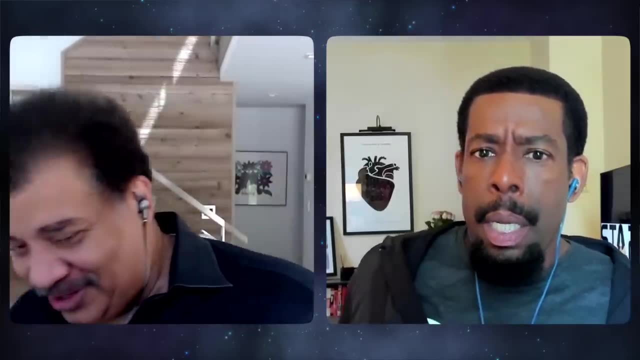 Quantum wedding crashing. That's it. We built this wall. You're supposed to stay out, Right? Did you see that potential barrier? Did you see that wall? Doesn't potential barriers mean anything to you? This would be good for Trump. 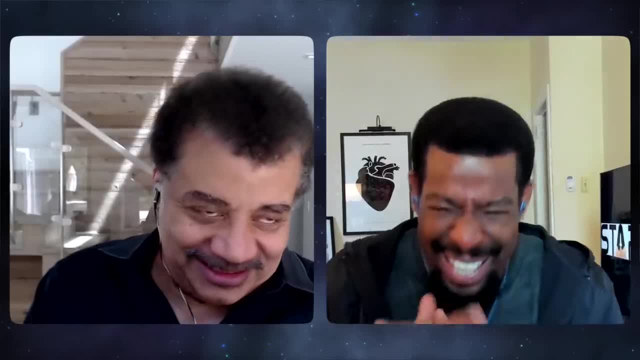 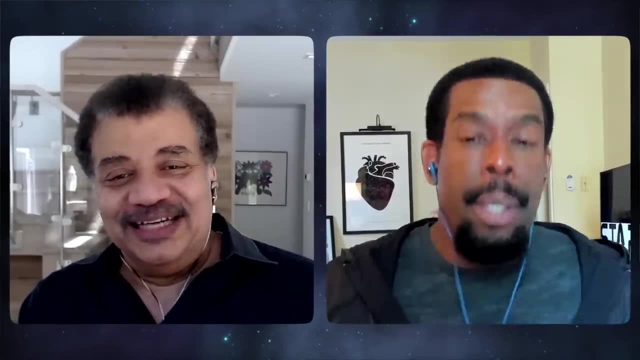 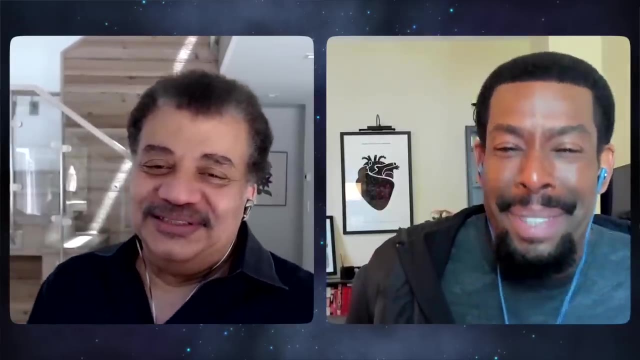 They built the wall to keep you out, But they're still tunneling in. They must be quantum mechanical entities. This is the thing. Why aren't these? Why aren't these quantum From Norway? I'm sorry, I can't. 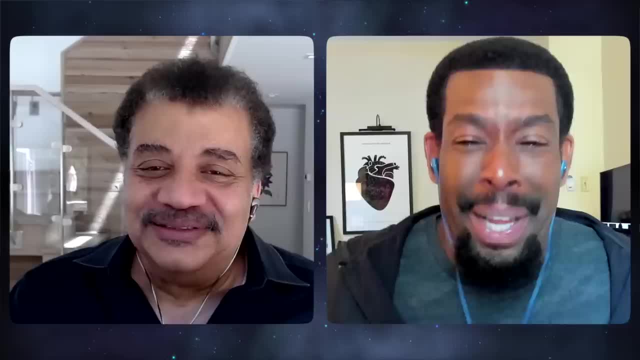 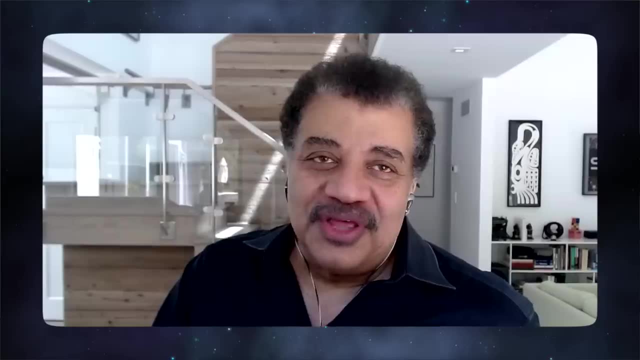 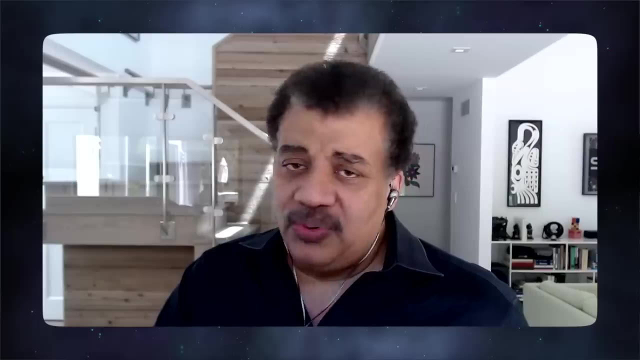 Why can't we get to what's from Norway? They wouldn't have to tunnel, Right? Okay, So that's just quantum tunneling, So here's. So I'll show you how that manifests Very interesting little history here, And then we'll call it quits, because this is just an explainer. 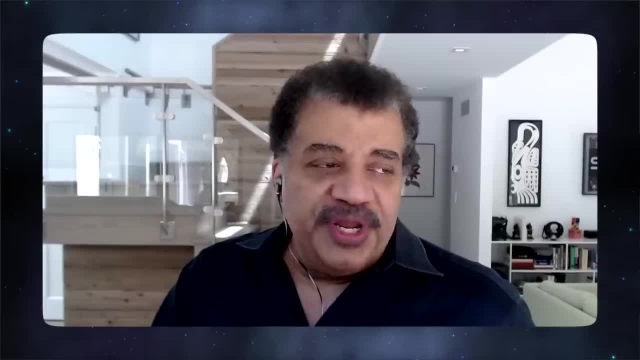 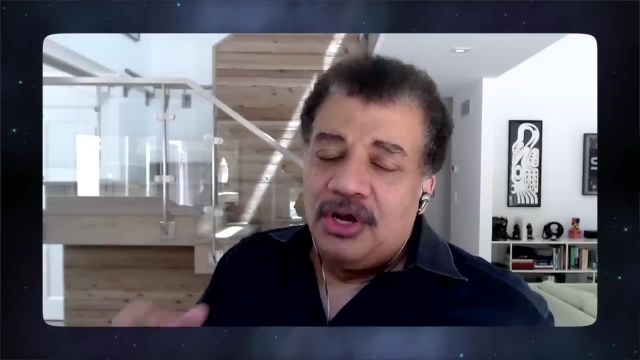 In the early days, a hundred some years ago, we didn't know where you got all the elements in the universe. Okay, By the way, I remember asking my high school chemistry teacher: where did the elements come from? Oh, they're in the earth. 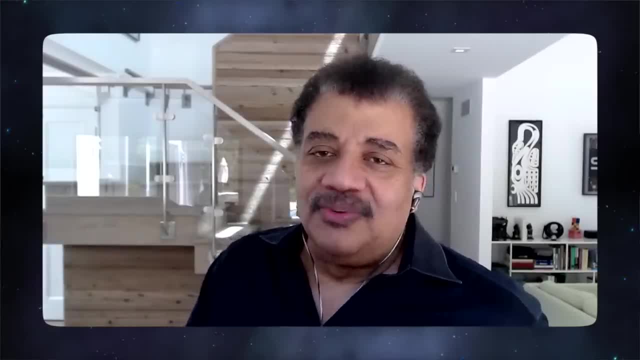 And I would later learn: No, we made these suckers and stars dude All right. Why don't you look up every now and then: Oh, that is so funny. Okay, So it's not his fault, He's a chemistry teacher. 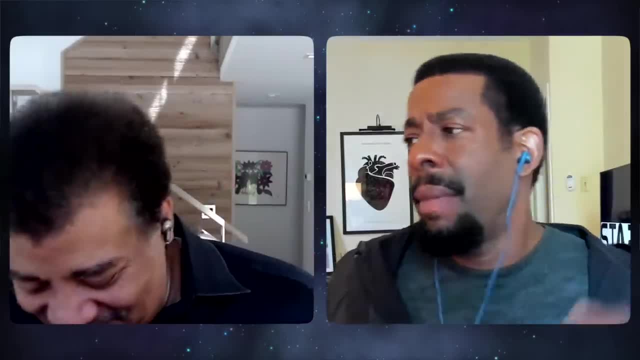 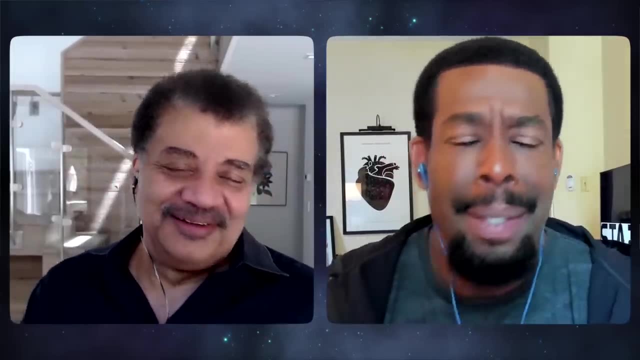 He thinks of the elements, And we know how stupid they are. No, Chuck, Come on, Let's be honest, He's a chemistry teacher. He's no physicist. Come on, What do you want, Chuck? What do you want? 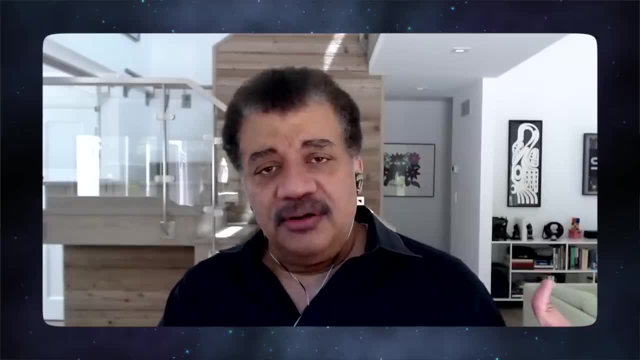 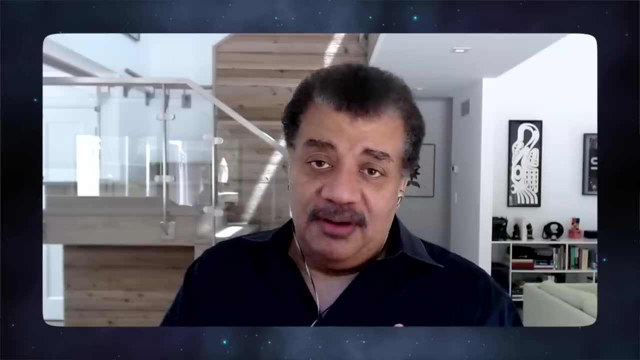 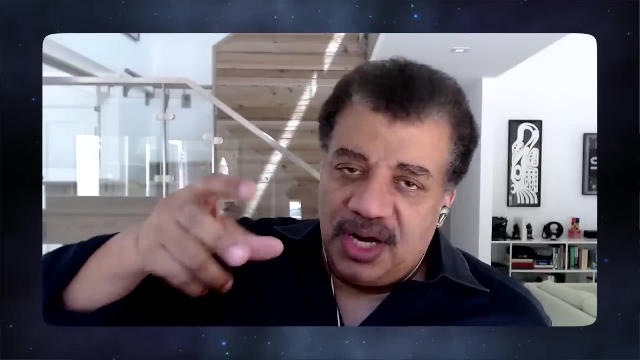 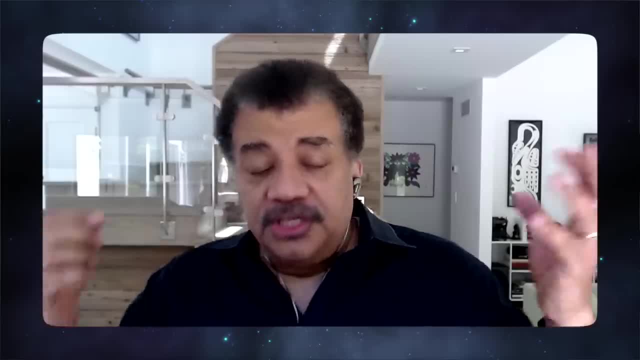 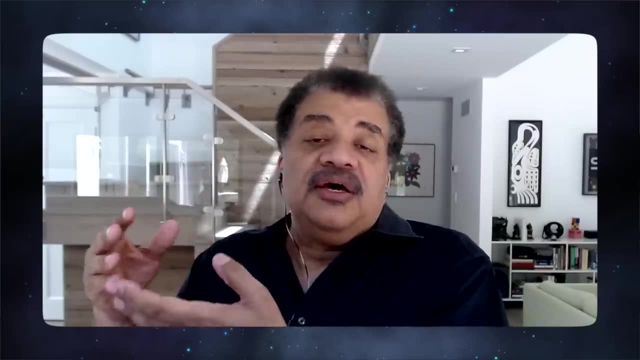 Okay, Now what's in the nucleus of a hydrogen atom? A proton. So you have a proton here and a proton there, And I want to merge them to make a nucleus that has two protons in it, which would be helium. 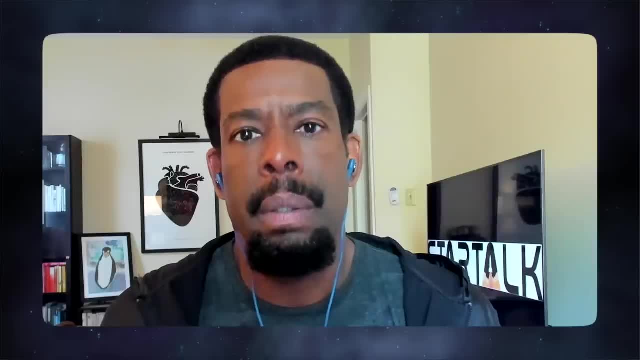 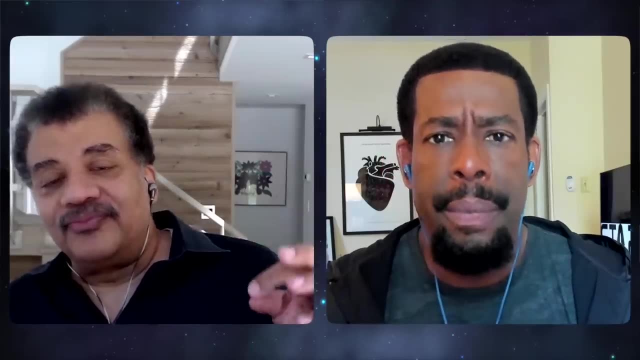 That's a way to build elements from scratch, Okay, Okay, So a proton is what charge? Wait, The proton is positive, Positive, Positive, And the charge on the other proton, It's also positive, It's also positive, Like charges. 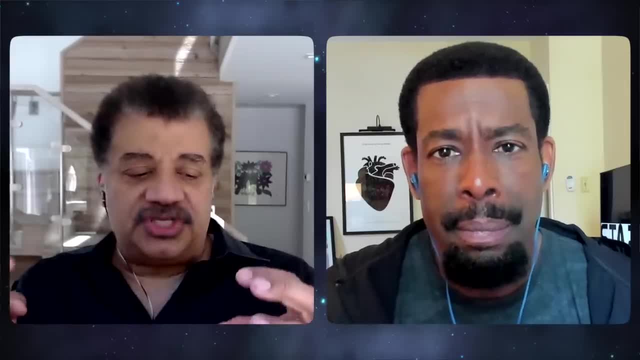 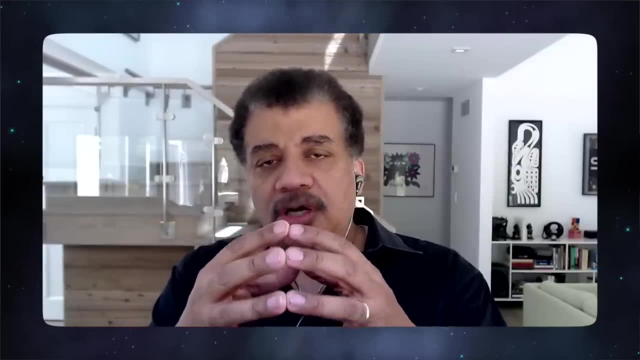 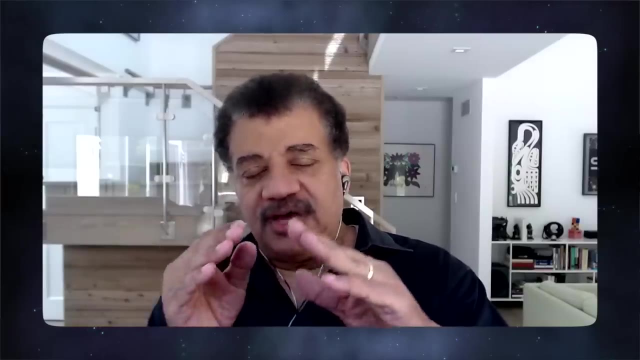 Oh, they don't really like each other. They repel. Okay, So you have to get them close enough so that a strong nuclear force kicks in and holds them together. Okay, That's the basic task you have to accomplish here. Sounds like Thanksgiving dinner at my crib. 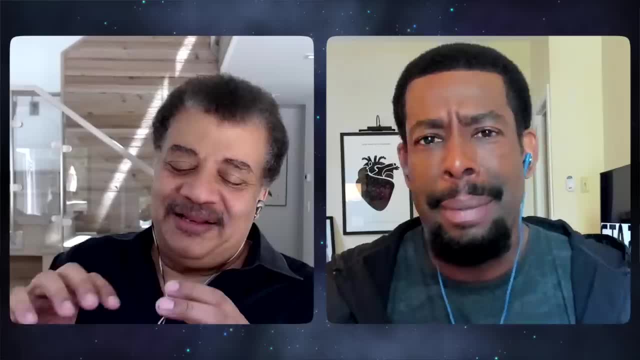 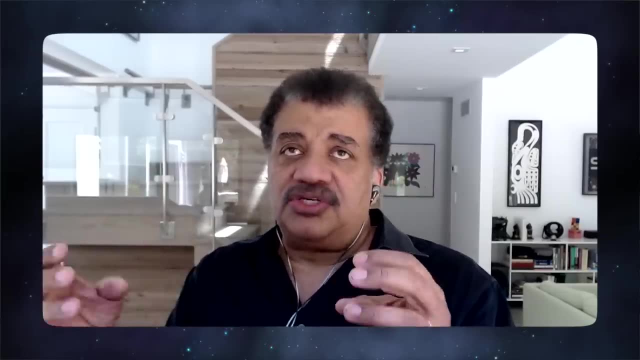 To force it in Right, Like, get in there, Get in there Right. So it turns out the electromagnetic repulsion, the two positive charges. you can sort of get them closer and closer if you speed them up by increasing the temperature of the plasma. 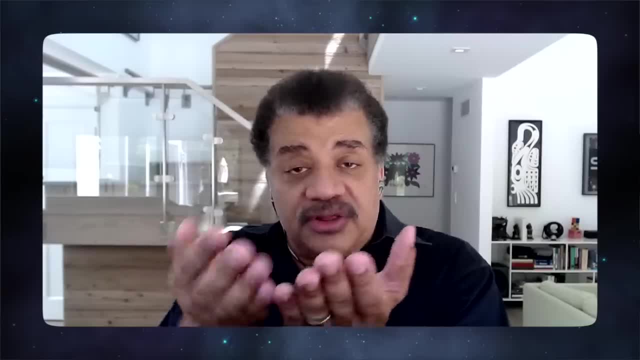 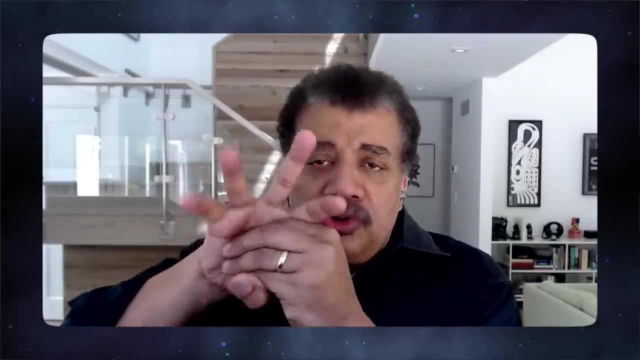 They'll speed up. They'll get closer and closer and closer to each other as you increase the temperature. Okay, Gotcha. So you ask: at what temperature will they be close enough for the strong nuclear force to kick in and grab them? 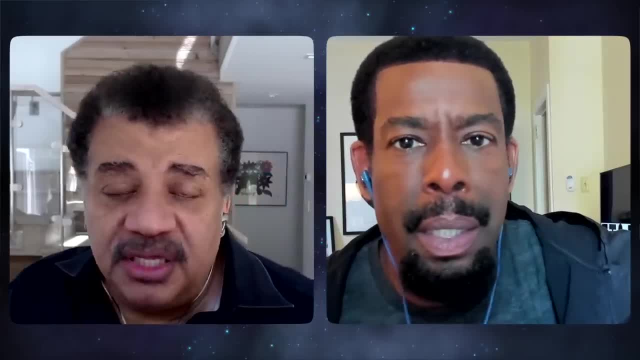 Okay, That's the question. Okay, That's the question. Okay, The temperature's like a billion degrees. Well, there you have it, A billion, And we look and we do the calculation for the centers of stars. It's not a billion degrees. 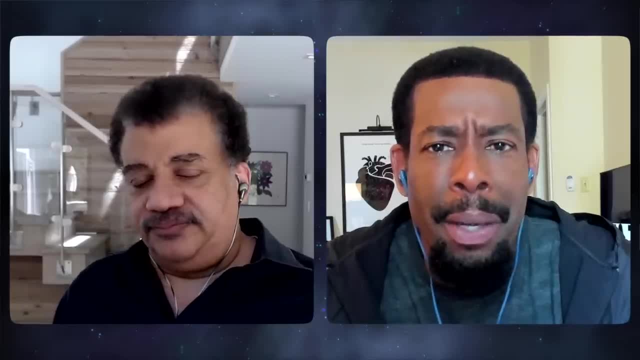 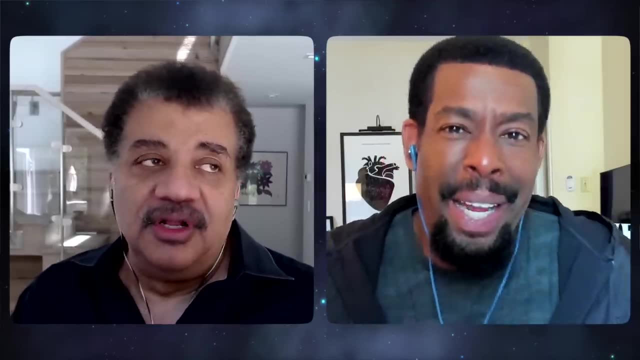 So I'm taking it that the building of the elements doesn't work by getting a billion degrees? No, it would if you could, If you could. But I'm saying that yeah, Right, Right. So the question was: so I think it was Eddington, a famous physicist of the day, astrophysicist. 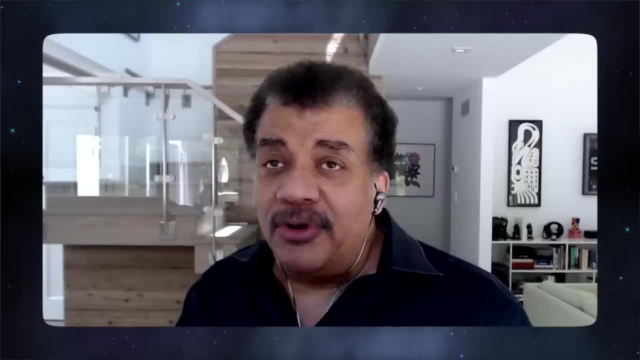 he was asked. he said: well then, Where are we going to get the elements? He says I don't know where, but if it's going to happen anywhere, it's going to be in the center of stars, Okay, 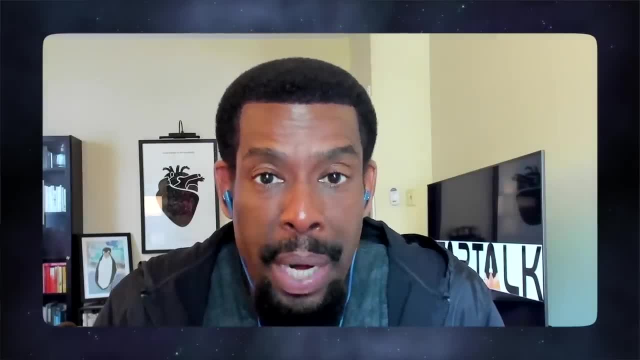 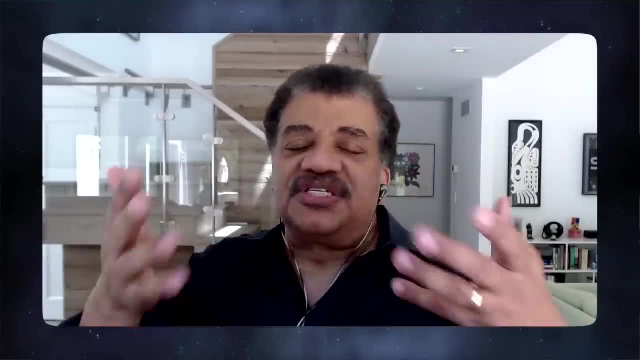 So even though we couldn't give him a billion degrees, he still said: I don't see any place else in the universe that will satisfy the needs of this requirement except the centers of stars. Okay, So there it just sat for decades. 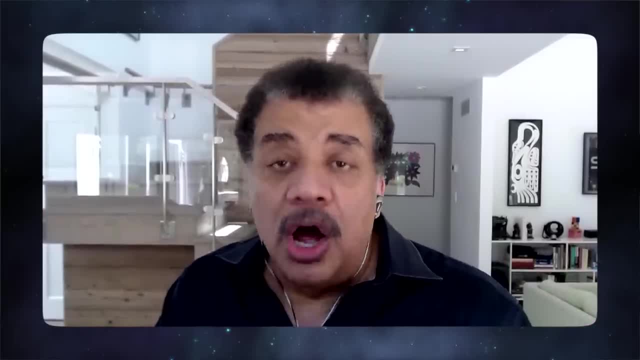 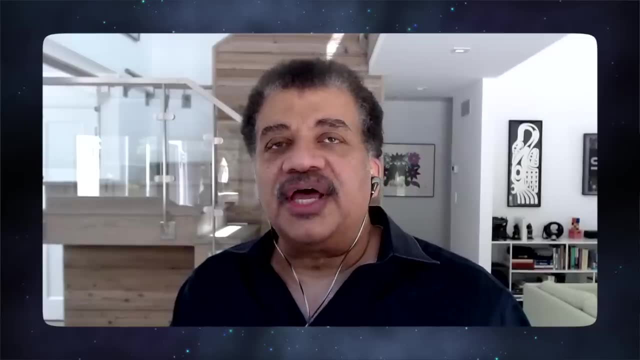 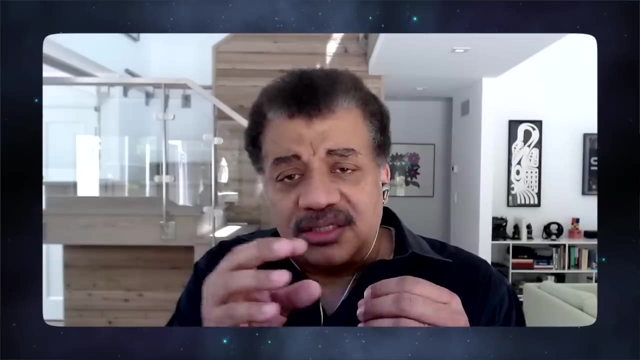 Okay, Not many decades, but it just sat there as an unsolved problem until quantum physics came along, And then they said: okay, here's a proton coming close to another proton, so there's a barrier there that it can't cross. 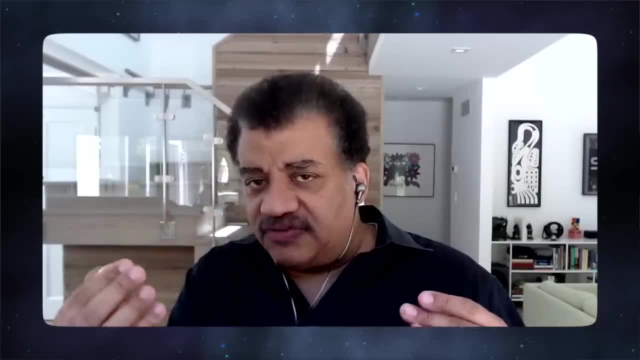 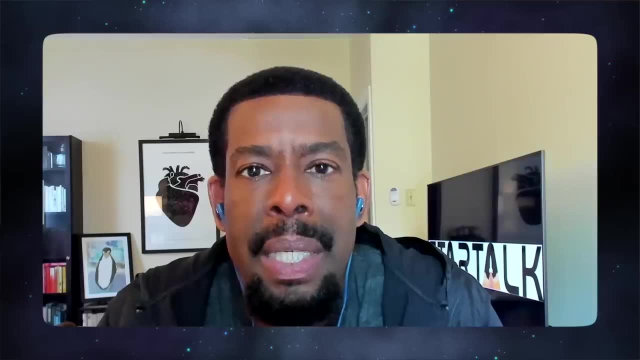 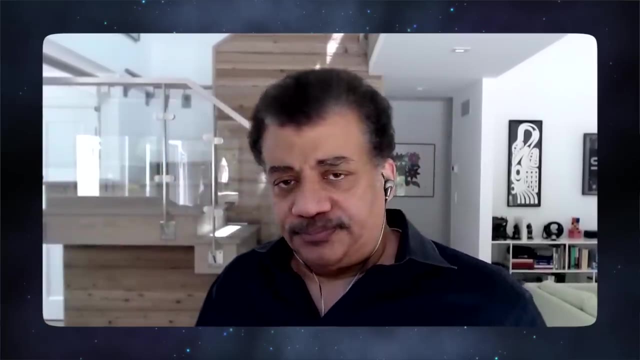 But wait a minute. the particles are also waves, and part of that wave exists within the grasp of the strong nuclear force Right, And so there's a probability that some of these particles will merge and make helium. Wow, So then you say: what is that probability? 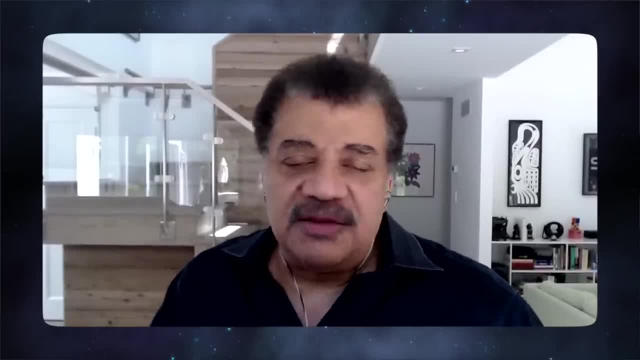 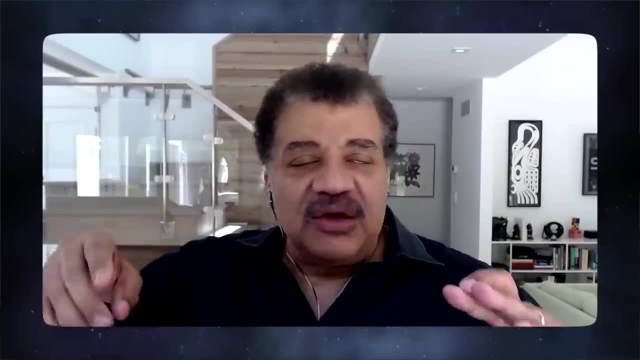 So they said: well, what is the temperature of the center of the star? They said 10 million degrees. It's not a billion, It's like 10, 15 million. So you do the math on the quantum physics and you say what percentage of collisions? 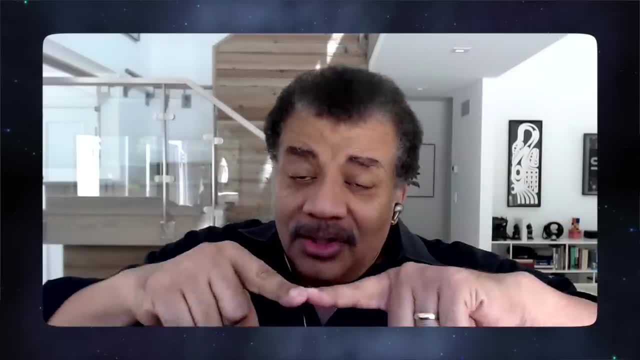 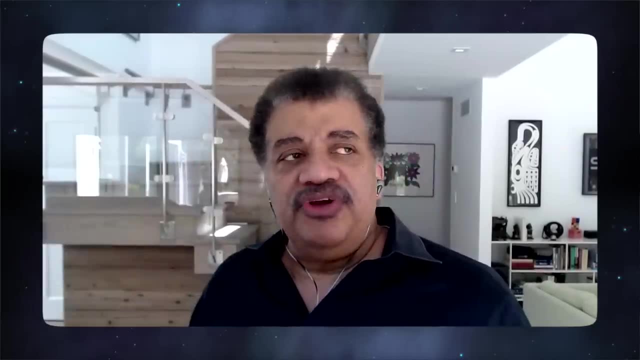 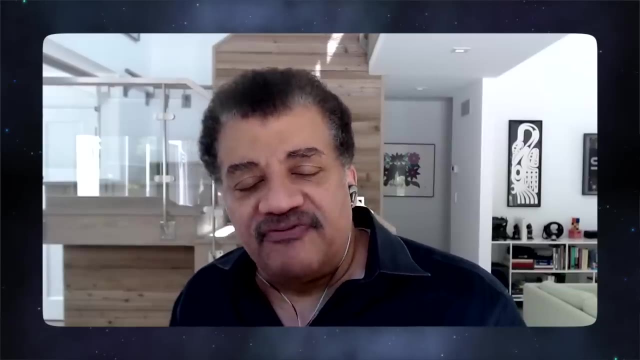 will tunnel through this barrier and end up making helium. You come up with that percent and, bada-bing, you recreate the total energy output of the sun. Look at that. So you're glad it's not converting every encounter into energy. 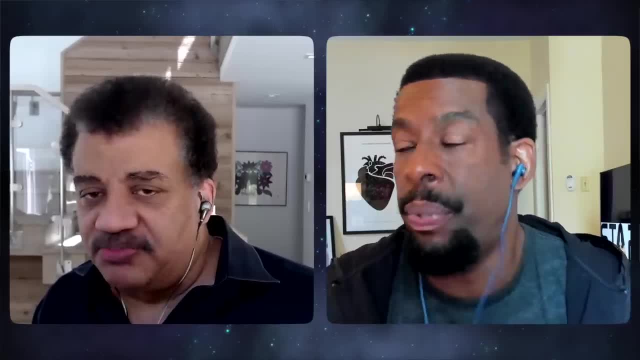 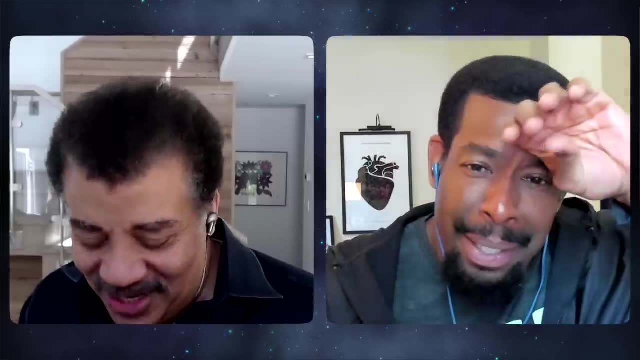 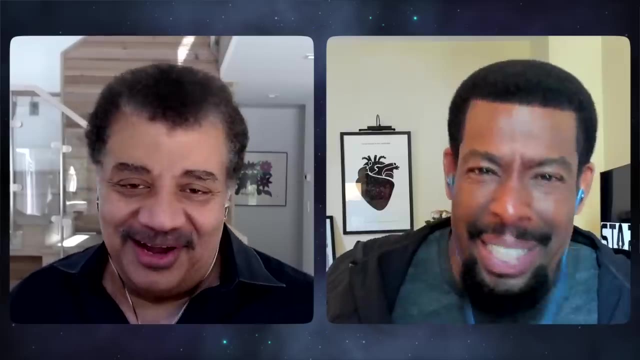 Right, The sun would just blow its smithereens. Well, yeah, Yeah, it's just like. why is everything, god damn, is hot, Says the person who, by then, is just a puff of smoke. Exactly, You don't have time to utter those words. 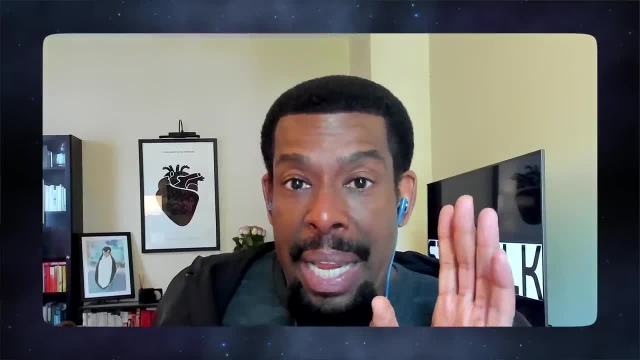 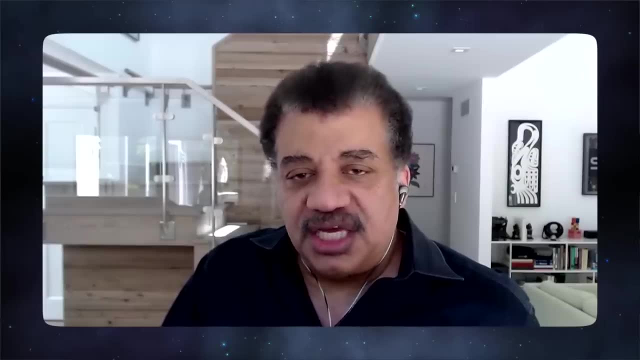 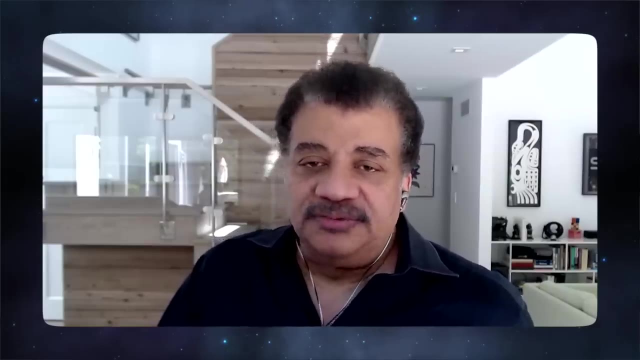 Right, Wow, Okay, that All right. Fascinating, Fascinating, All right. So the thermonuclear fusion in stars that generates the energy at the temperatures it does can only happen because of quantum mechanical tunneling. That's boom, that is amazing. 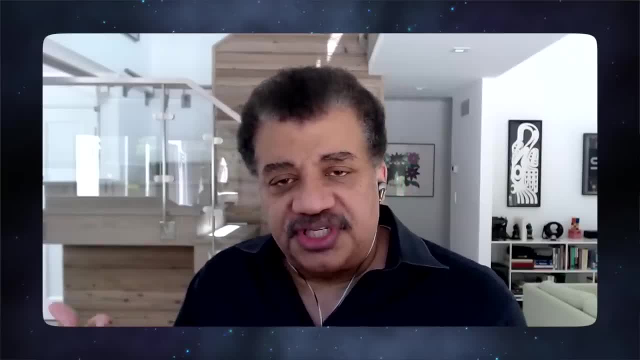 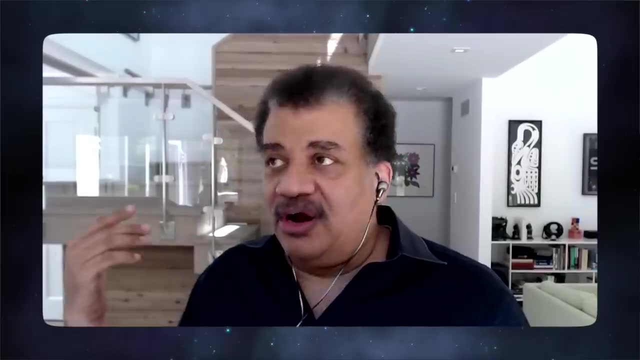 And so just think about the challenges we astrophysicists have. We have an idea And, by the way, so Eddington was right- It does happen in the centers of stars, Of course. Right, Because nowhere else was rational, right. 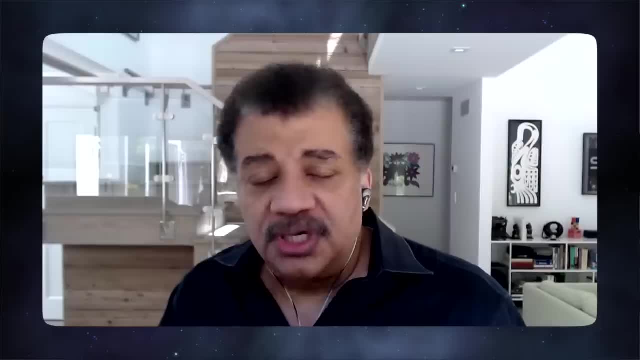 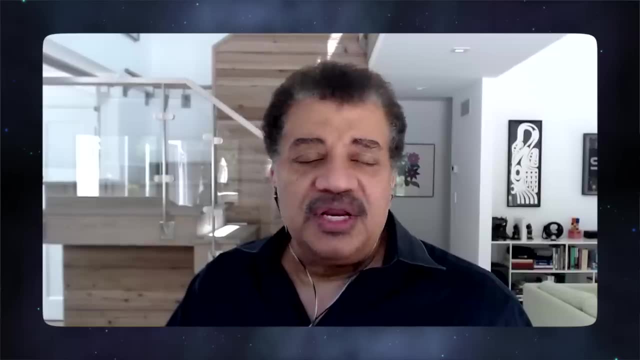 Right, But we didn't know. We didn't know enough physics at the time. it was proposed to answer that question. New physics had to be invented, And this is why we are always so excited when new physics comes along. There are people who say: people say, oh, someone has a new physics idea. but everyone. 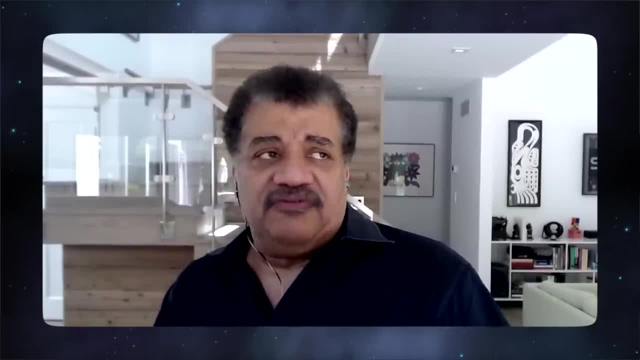 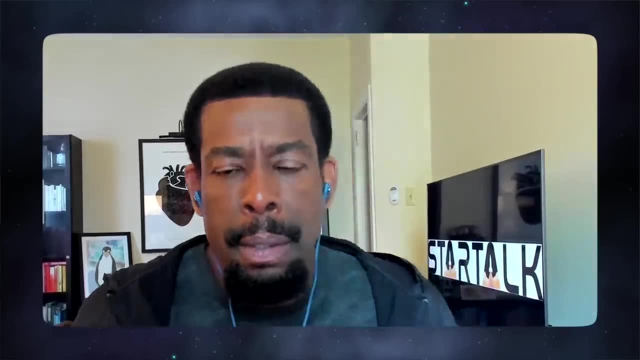 else is rejecting it because they don't want to lose their highly invested lives in this. They're thinking that we don't like new ideas. They got to you, Neil. We love new ideas. Yeah, Because they give a whole new idea. 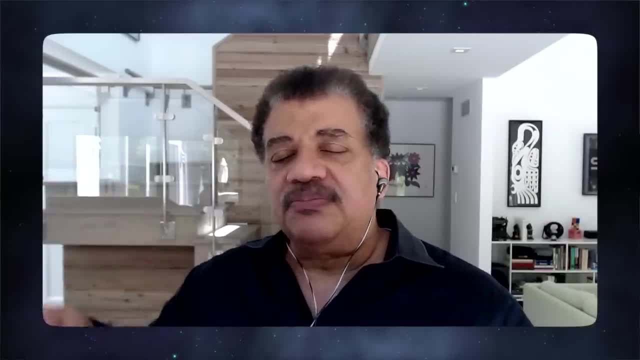 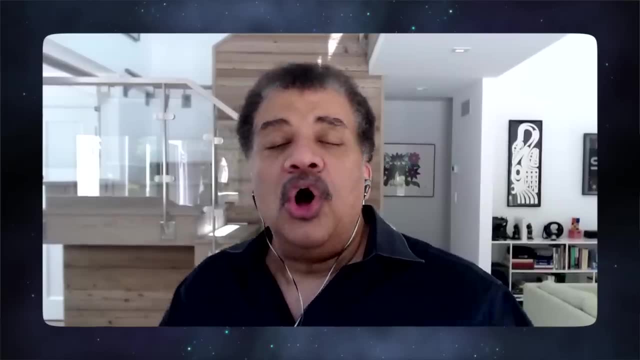 They give a whole new understanding on the frontier of stuff that we didn't previously understand. And so, yeah, that's quantum mechanical tunneling. Oh, oh, one other thing: It no matter the size of that potential barrier, Right? 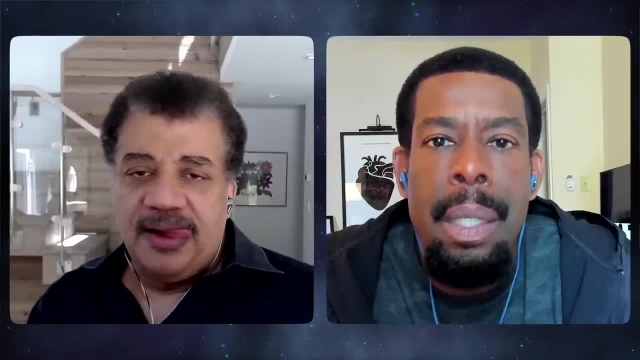 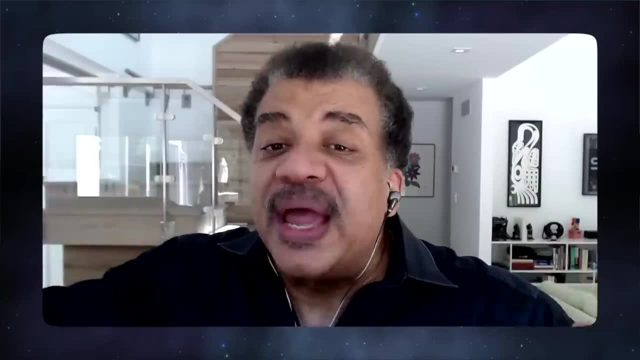 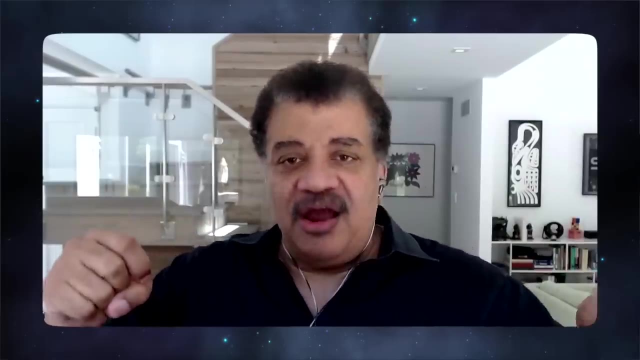 It tunnels and appears on the other side instantly. Oh so, okay. So The wave function just collapses and it's there. Right, It doesn't travel there, It was always there, probabilistically, Okay, Okay. So when your wave becomes the particle boom, it is there. 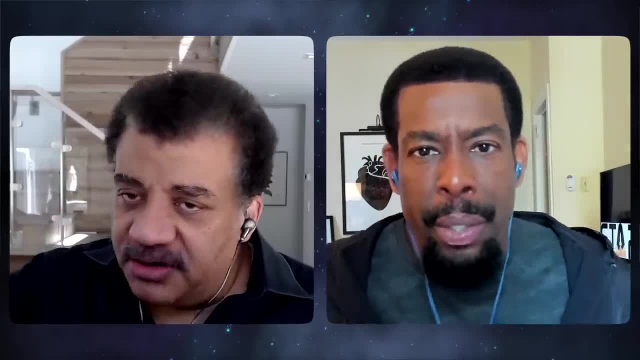 So then, distance makes no, it's immaterial, It's immaterial, It's immaterial, It gets, it's instantaneous, It's instantaneous. So we think that it moved, but it really didn't. It was always there to begin with.